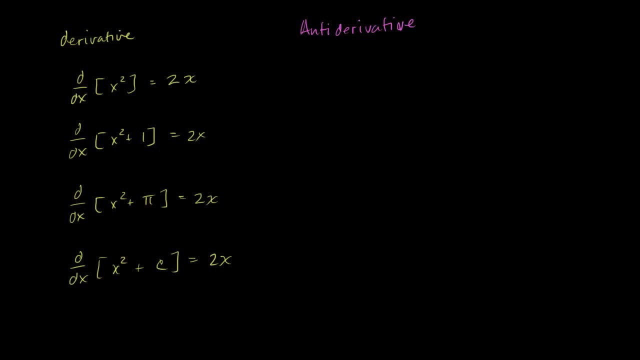 we want to find what it could be the derivative of. So if someone were to tell you or give you 2x, if someone were to say 2x, let me write this. So if someone were to ask you, what is 2x? the derivative of, they're essentially: 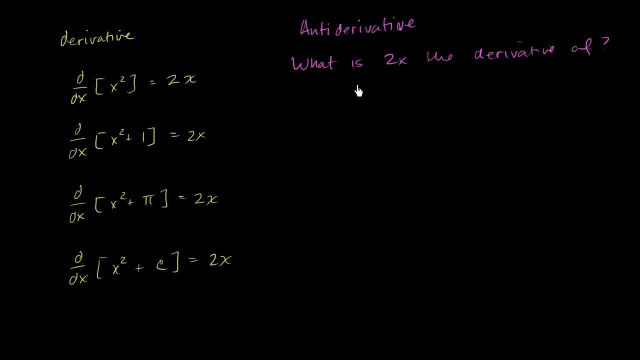 asking you for the antiderivative, And so you could say: well, 2x is the derivative of x squared, x squared. You could say 2x is the derivative of x squared. But you could also say: 2x is the derivative of x squared plus 1.. 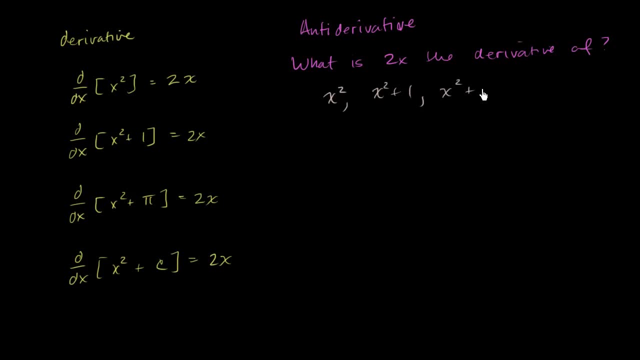 You could also say that 2x is the derivative of x squared plus pi. I think you get the general idea. So if you wanted to write it in the most general sense, you would write that 2x is the derivative of x squared plus some constant. 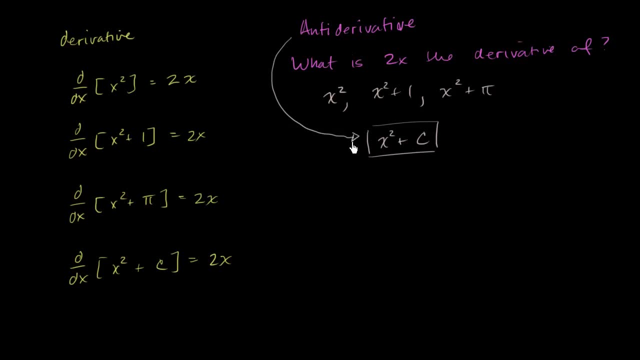 So this is what you would consider the antiderivative of 2x. Now that's all nice, but this is kind of clumsy to have to write a sentence like this. So let's come up with some notation for the antiderivative. 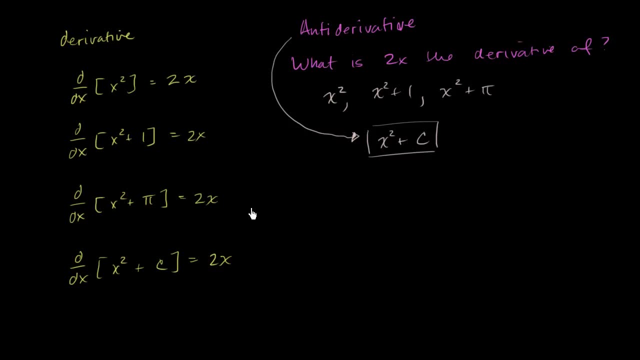 And the convention here is to use kind of a strange-looking notation- is to use a big elongated s-looking thing like that and a dx around the function that you're trying to take the antiderivative of. So in this case it would look something like this: 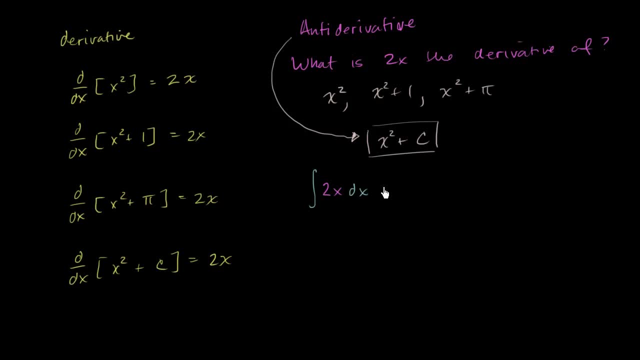 This is just saying this is equal to the antiderivative of 2x. And the antiderivative of 2x- we have already seen- is x squared plus c. Now you might be saying: why do we use this type of crazy notation? 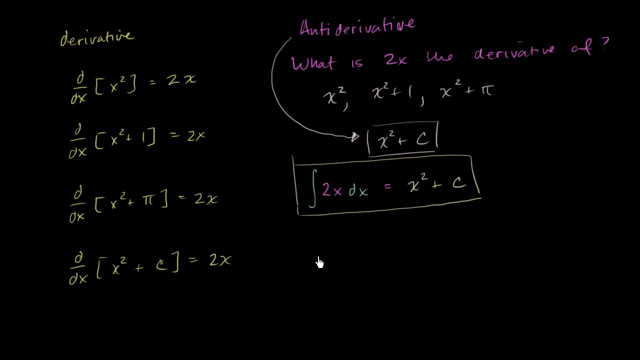 It'll become more obvious when we study the definite integral and areas under curves and taking sums of rectangles in order to approximate the area of the curve. Here it really should just be viewed as a notation for antiderivative And this notation right over here, this whole expression. 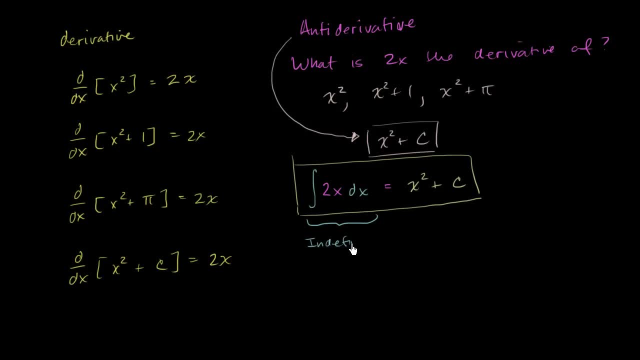 is called the antiderivative of 2x, The indefinite integral of 2x, which is another way of just saying the antiderivative of 2x.